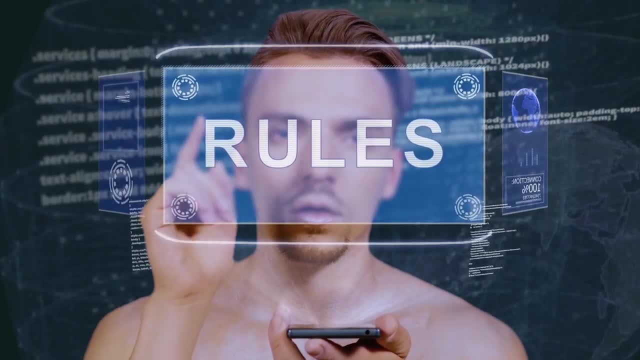 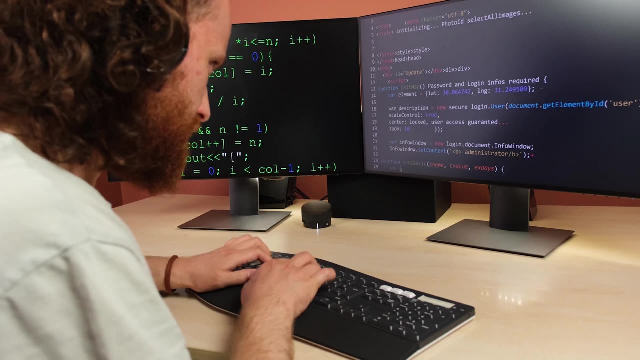 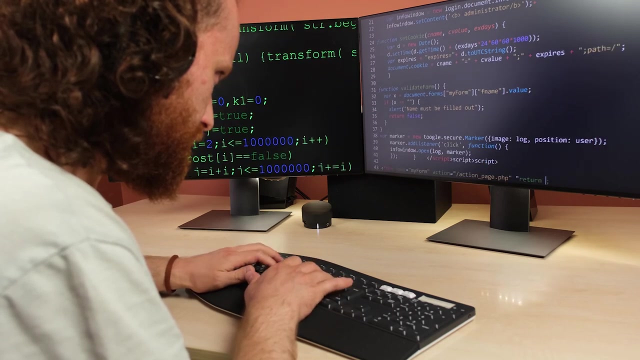 will arise if you ask 10 persons to complete the identical program. they will each complete it in their way. So programming paradigms are different techniques for writing your program. It is critical to understand how we will write a program Understanding the programming paradigm. 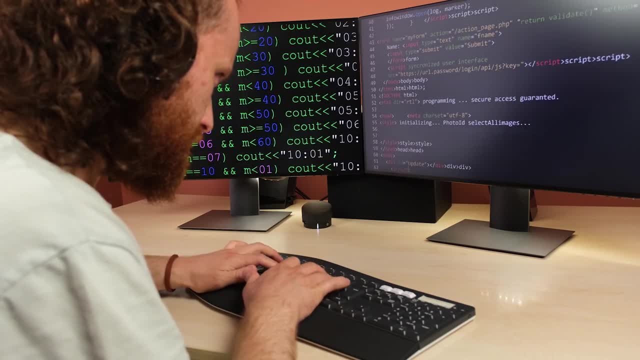 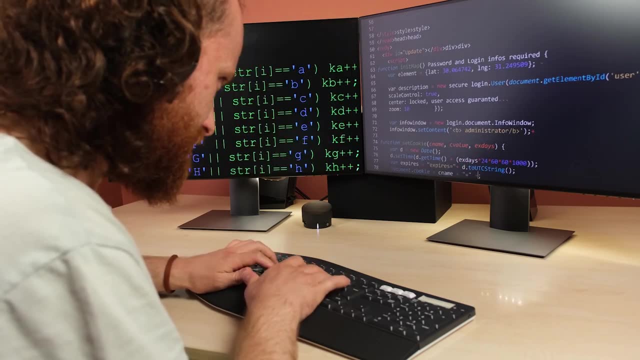 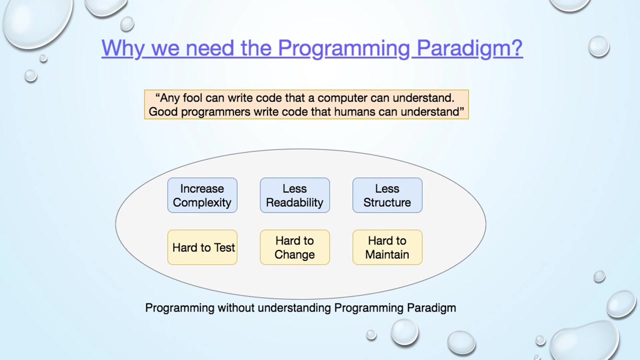 is necessary for that. When selecting a programming language for building a program or software, we must ensure that it supports the programming paradigms. Why do we need a programming paradigm? One of my favorite coding quotes is: any idiot can create code that a machine can understand. 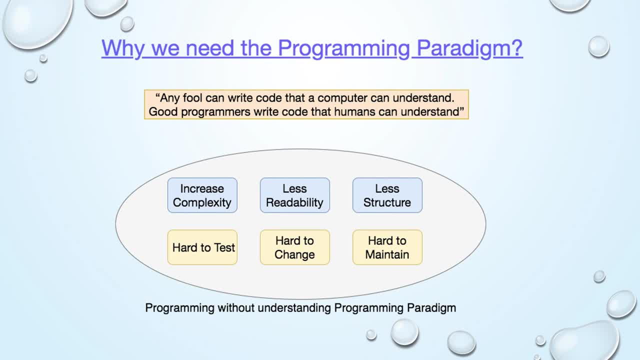 skilled programmers produce code that humans can understand. Consider building software with 10,000 lines of code with a group of people. What happens if they all create the software in their style? First and foremost, the program's complexity will rise. The program's readability and structure will suffer. It will be tough to test and updating. 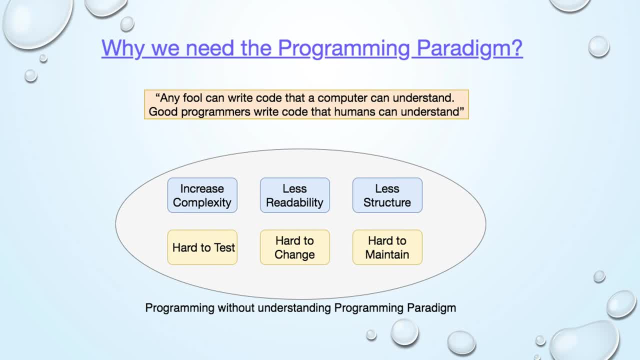 the code will be incredibly complex. What will happen if everyone writes your application using a set standard? We can reduce many of the problems. A programming paradigm will assist us in resolving all problems. Thus, the programming paradigm offers a unique standard for developing programs or software Types of programming paradigm. 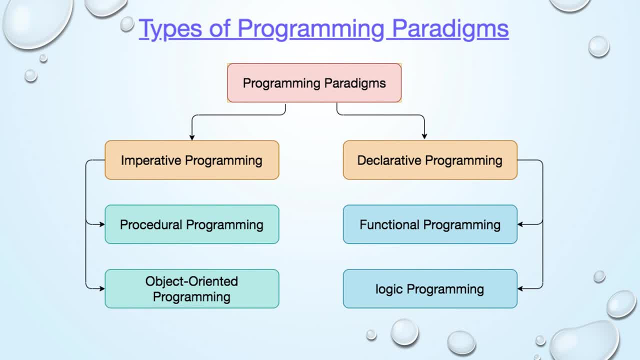 The two sorts of programming paradigms are imperative programming and declarative programming. The two types of imperative programming are procedural and object-oriented. There are two types of declarative programming: logical and functional. Let us examine each of these points in further depth. 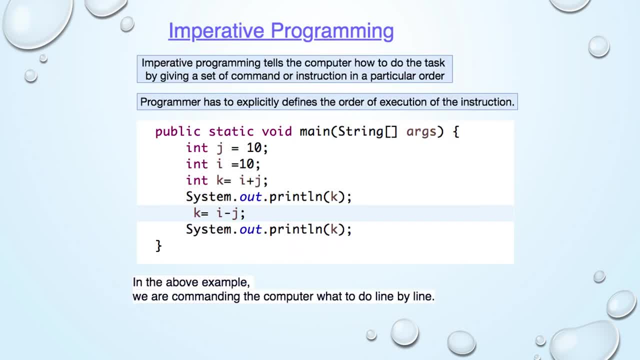 Imperative programming. The word imperative implies command. Imperative programming tells the computer how to complete a task by giving a list of commands or instructions in a specific order. The order of instructions is significant in imperative programming. In this example, we are giving the computer 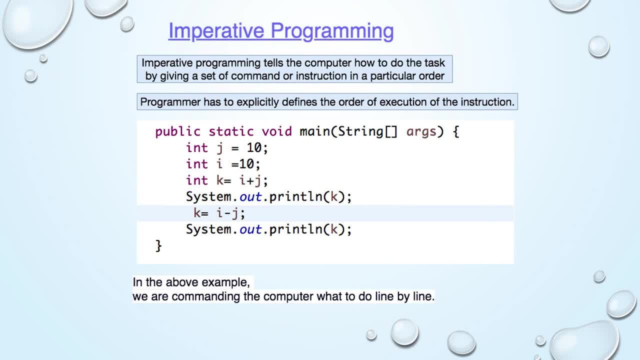 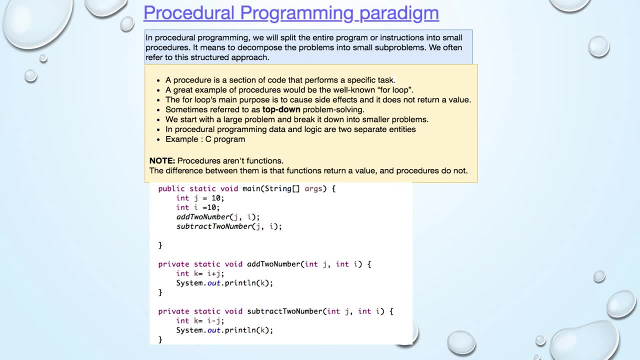 line-by-line instructions on how to add to numbers and subtract to numbers. Procedural programming. In procedural programming we divide the problem into smaller subproblems. We often refer to this structured approach. A procedure is a chunk of code that performs a specified task. Data and logic are separate entities in procedural programming. 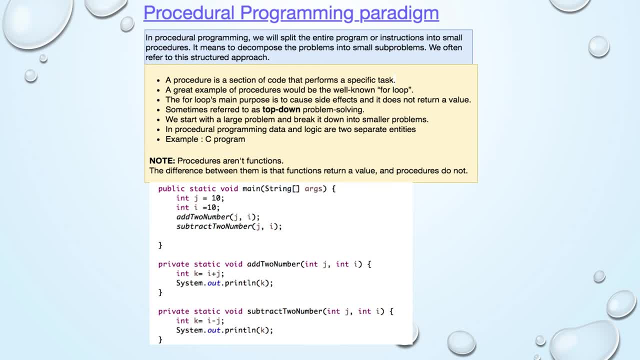 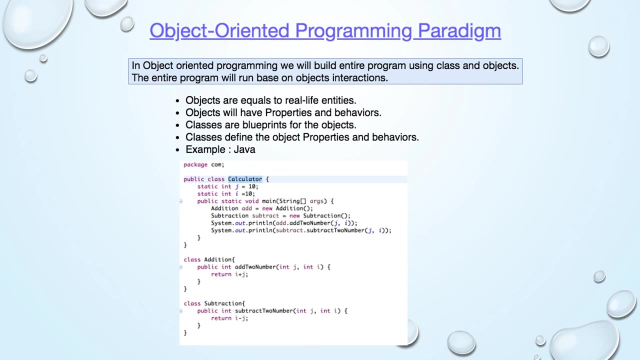 Here we have two procedures: add to numbers and subtract to numbers. The main procedure will call this sub procedure to add and subtract numbers. Object-oriented programming. In object oriented programming we will use classes and objects to create an entire program. The whole program will run depending on object interactions, Objects. 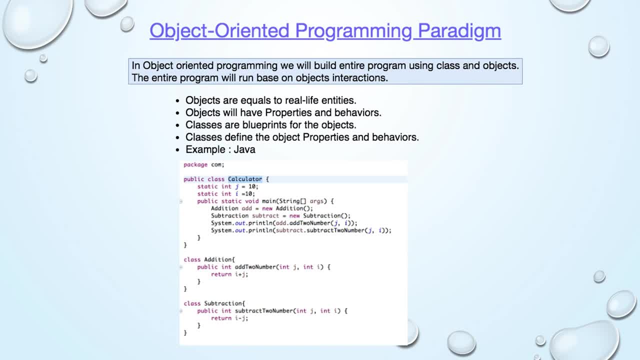 are real-world entities with properties and behavior. The classes act as the object's blueprint. Classes describe the characteristics and behavior of objects. In this example you can see that we have three classes: Calculator, Addition and Subtraction. The Addition class is in charge of adding to numbers. 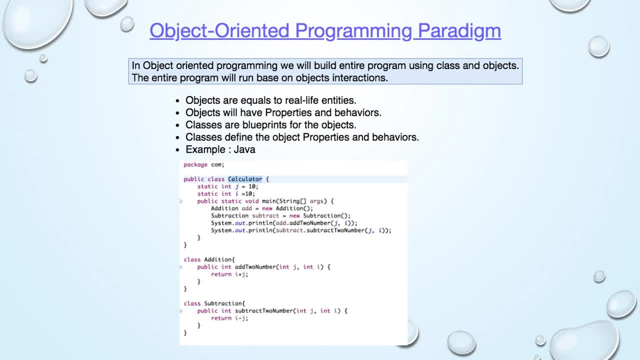 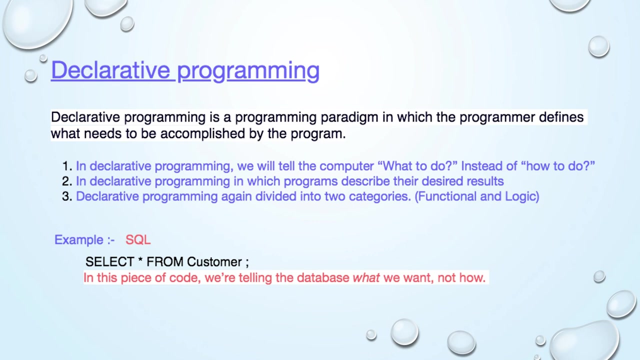 The Subtraction class is in charge of subtracting to integers, So the Calculator class will call the Addition and Subtraction classes to add and subtract to numbers. Here all three classes interact to produce a result. Declarative Programming. In declarative programming we tell the computer what to do, rather than how to do it. 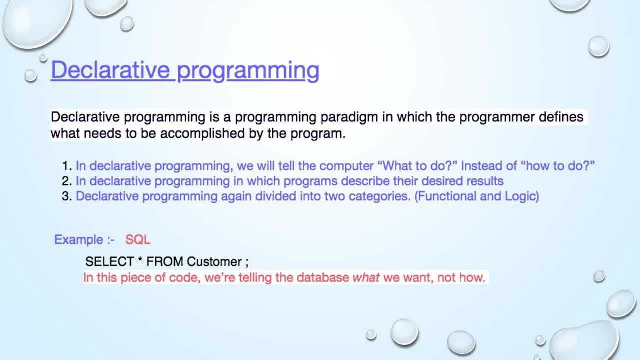 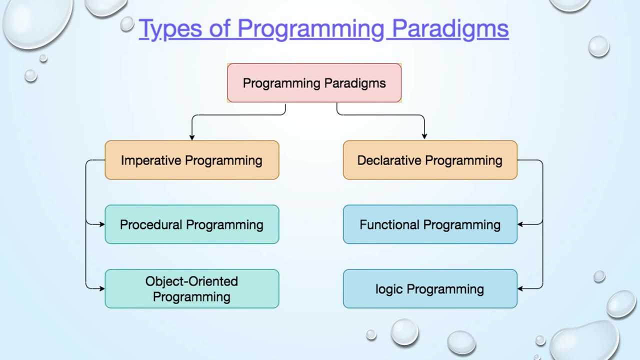 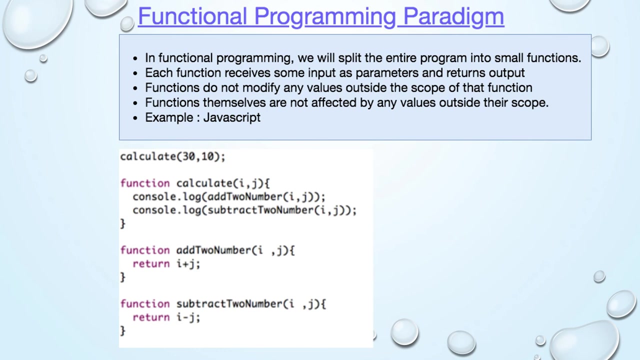 We shall always focus on output or result in declarative programming. In this sample code, we are telling the database what we want rather than how it should do. Functional and logical programming are the two main subtypes. Functional Programming: In functional programming we will split the entire program into two functions. 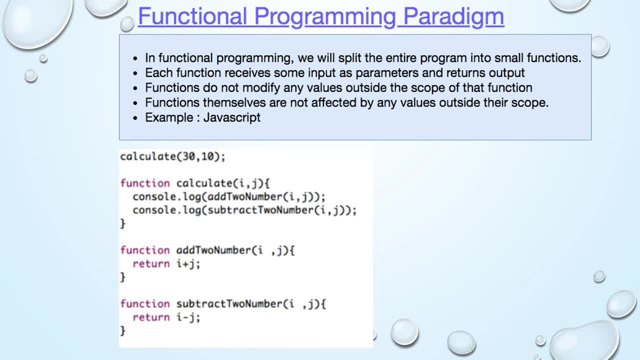 Each function takes some parameters as input and returns the output. JavaScript is one example of a functional program. Here in the example we have three functions: The AddToNumber function adds to integers. The SubtractToNumber method subtracts to integers.